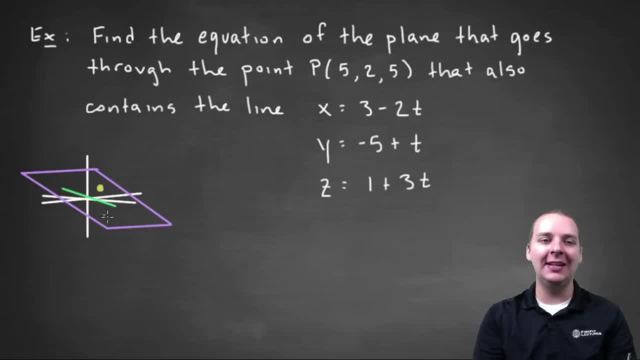 it runs inside of that plane. This line is contained inside of the plane here, and that's the line: X equals three minus two T, Y equals negative five plus T and Z equals one plus three T. here Now, when you, you know, think back to when we were talking about equations. 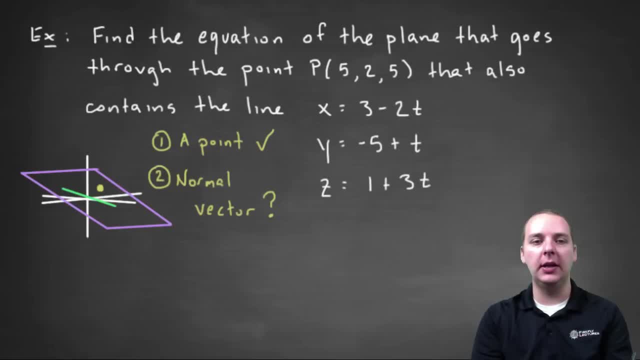 of planes. we needed two things: to write the equation of a plane down, We needed a point in the plane, any point in the plane which we, which we have provided to us. and then we also needed a normal vector for the plane, That that was a. a vector. that meant that 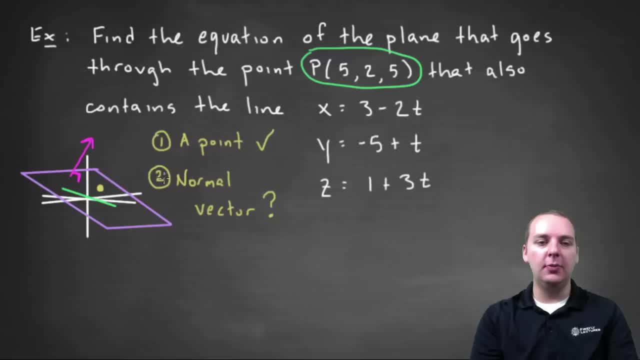 we need to set the plane at a right angle. Now, to me, that seems to be the thing that's missing. Now, when you look at this line, there is a vector that's related to this line. You remember when we were discussing a, a line in space, there was a, a vector that came. 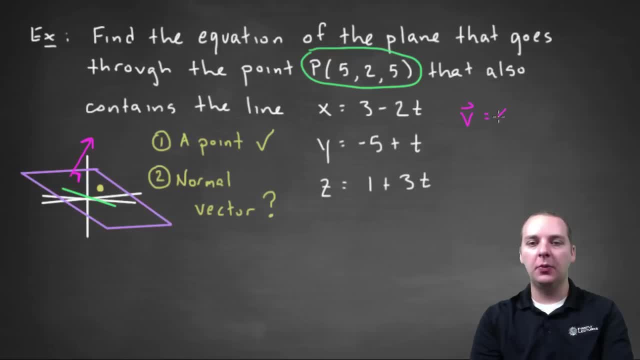 into question the vector ABC, which in our case is negative. two comma one comma three. This is X naught plus A, T, Y naught plus B, T, Z naught plus CT, as you know, and the vector ABC was a direction vector for the line. 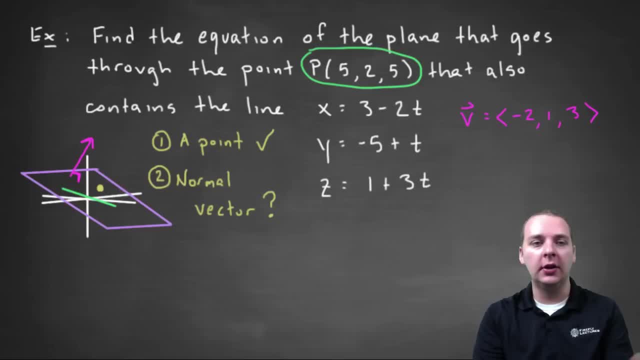 So that's a vector. I don't know if that's the one we need or not, but it was a vector. And so if you look, that line has a direction vector like this. But you notice that vector is not orthogonal to the plane, it's inside of the plane. 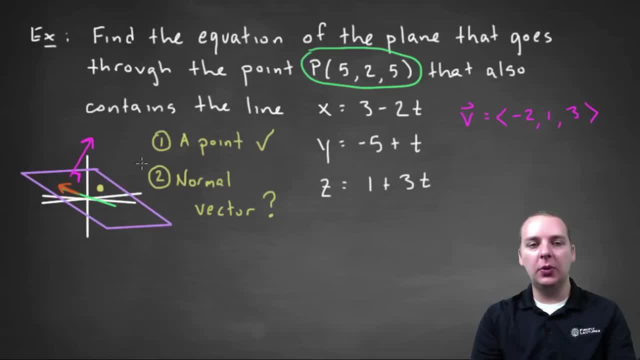 It doesn't meet the plane at a right angle. So this is the one where I'm really getting stuck. So I'm going to ask you a question: how on earth do you think we can find a vector with the information that's been given to us, find a vector that is orthogonal to our plane? 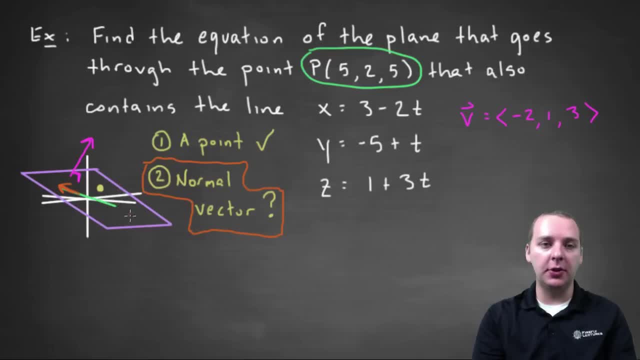 Pause the video if you need to to think about it, but I'm going to share with you how to find this guy. Basically, what we're going to do is we're going to get this vector, similar to how we got it in the last video. 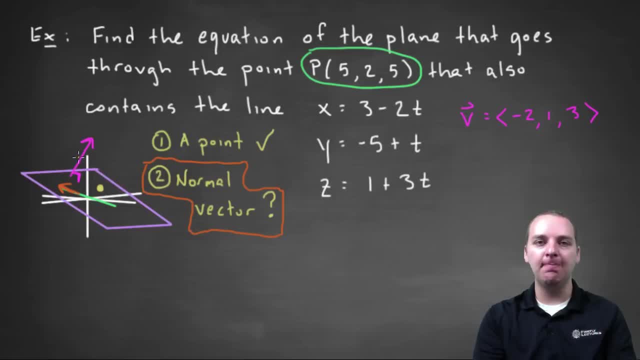 We're going to find two vectors that are in the plane. We already have one, by the way. This vector here is in the plane, but we need one other vector that's in the plane, And then we're going to take their cross product because, as you know, when you take the cross, 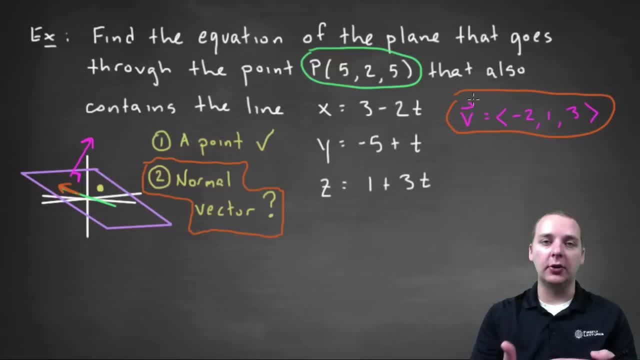 product of two vectors. it's going to give you a third vector, a new vector that's going to be orthogonal to both of the other two vectors, And so that would be the guy that we're after here. So one of our vectors is negative- two, one, three- but who's the other vector? 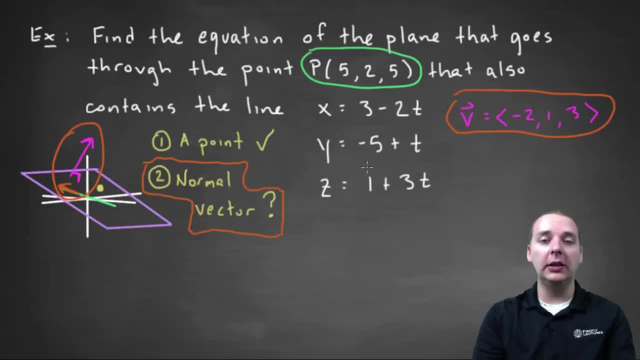 Well, this line here can reveal a lot, A lot of the different points that are on your line, a lot of the- I'm sorry, a lot of the points that are in your plane, because all the points on the line are in the plane. 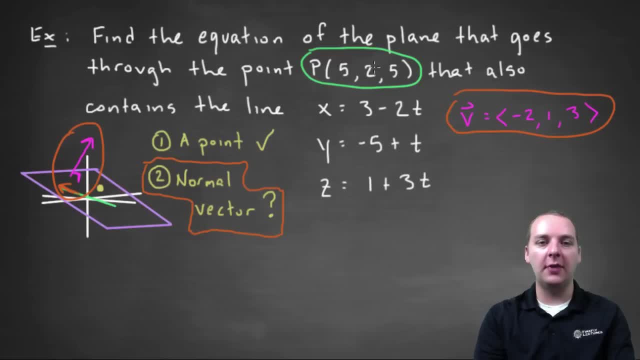 And then we also have another point in the plane, this five, two, five point here. So what? what can we do? Well, we're going to create a second vector in addition to this one that's in our plane from P to some point on the line. 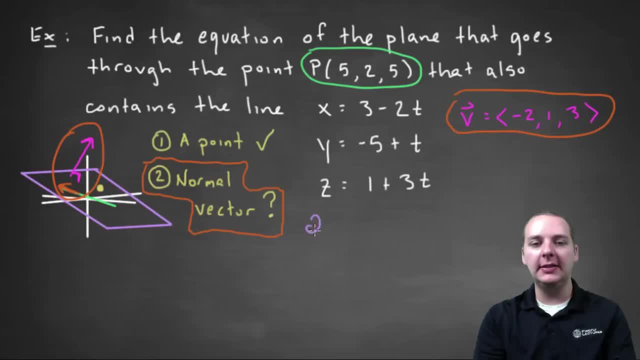 It doesn't really even matter what point that is Now. The second point that I can already tell is on my line is X naught, Y naught, Z naught, If you recall from when we were talking about equations of lines in space. 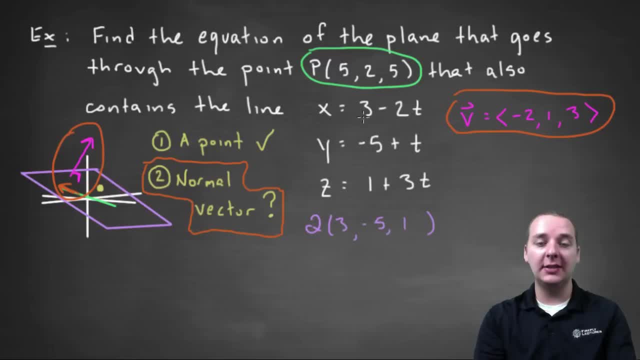 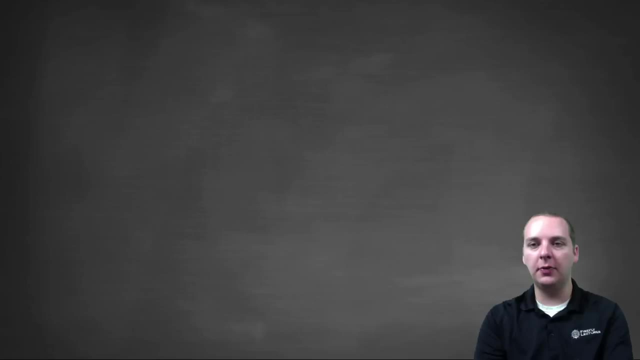 So three comma negative, five comma one. that's a point that's on our line And of course, as a result, that also means it's in the plane, since the line is in the plane, All right. So let me get rid of some of this stuff here and make some space so we can write a few. 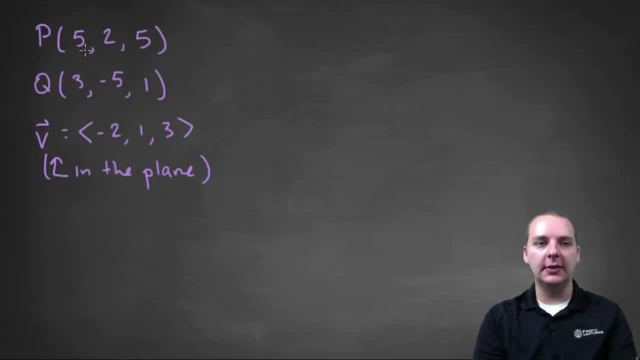 things down. All right, So I've I've copied a few of the things down. The point P was the five, two five point that was provided, The three negative five. one point was a, a point on the line. 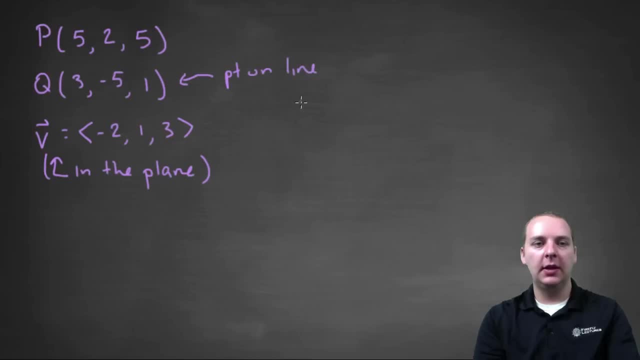 This is a point on the line. And then we have the vector V here: negative two, one, three, and that was the vector that was in the plane. So let's make also make sure we're keeping straight points versus vectors. 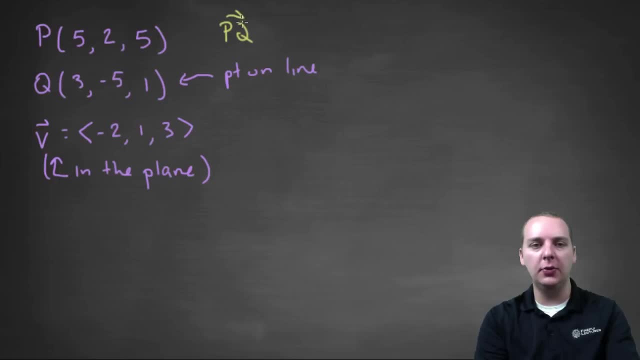 So first up, let's create a vector, We'll call it PQ. To do this, we'll write it in component form. and to, to change a line segment into a vector in component form, you'll do terminal minus initial. So three minus five is negative two for the ith component. 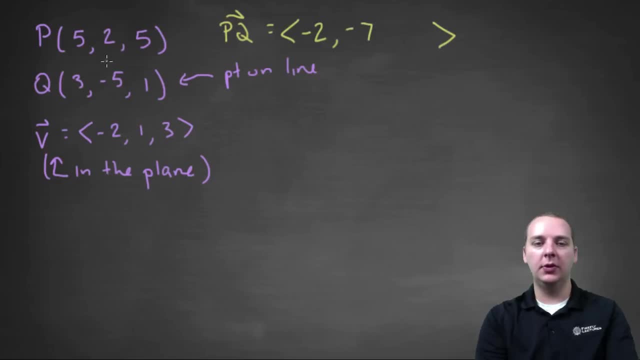 Negative five minus two is negative seven for the jth component and one minus five is negative four for the kth component. So this is a vector In the plane and this is a vector in the plane. So if you had a plane that looks something kind of like this, what we just found are 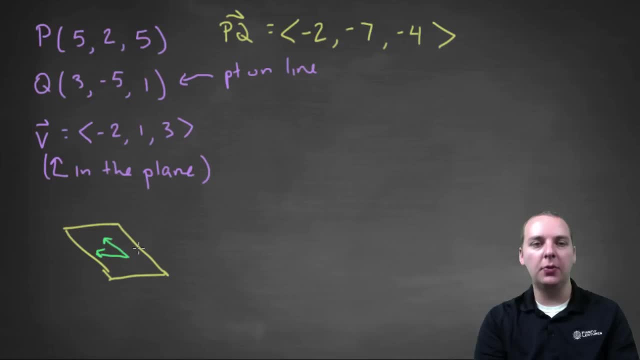 two vectors like this guy and this guy, for example, We just found two vectors, him and him, that are both in the plane, And what I'm about to do is take their cross product, which will give me a vector that's orthogonal to the plane. 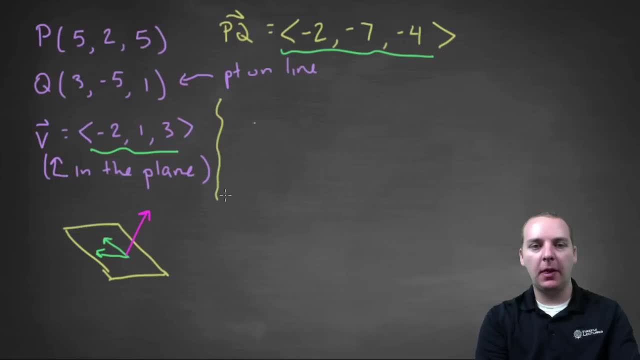 So let me see if I can squeeze that in here. Okay, We'll take PQ, cross V, which we'll get by taking a three by three determinate IJK, And then negative two, negative seven, negative four and negative two, one, three. 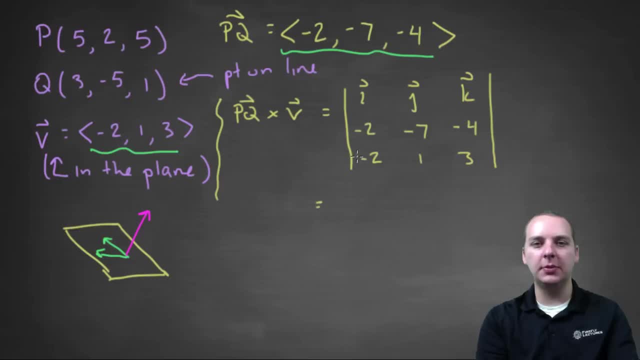 I'm going to skip some of the basic arithmetic algebra type stuff just to speed things along. The ith component will be negative three, It will be negative one plus four. negative twenty-one plus four, so that'll be negative seventeen I. The Jth component will be minus six minus eight. minus six minus eight, that'll be minus. 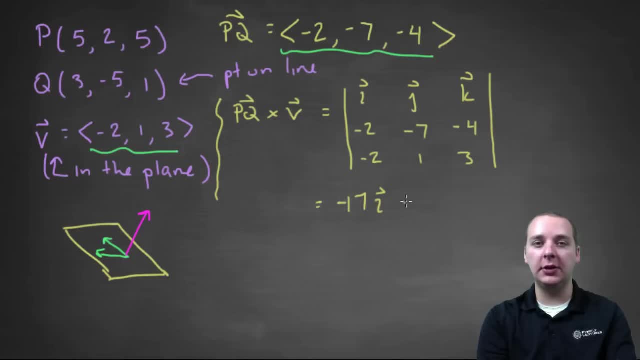 fourteen, But you remember the Jth component. you have to change the sign so it'll be plus fourteen J And then the kth component will be negative. two minus fourteen I. Okay, So that'll be minus fourteen, Okay, Okay. 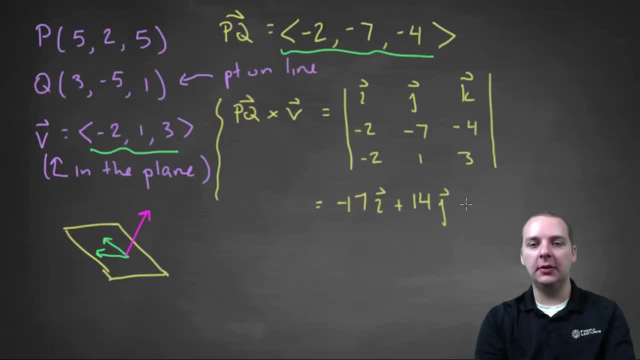 Okay, 14, which would be negative 16 K, And that guy is our normal vector to the plane. that was the one that was so difficult to find and we found it And the equation to the plane. this is going to be like our ABC normal vector for the plane. 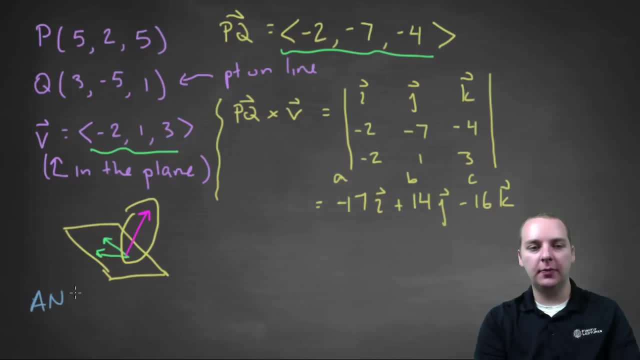 So we're pretty much done, just have to write down the final answer. So the final answer would be A X minus X naught, which would be negative 17, X minus some XYZ point. that's in the plane. You could take P or you could take Q, it doesn't really matter, I'll just take 525..